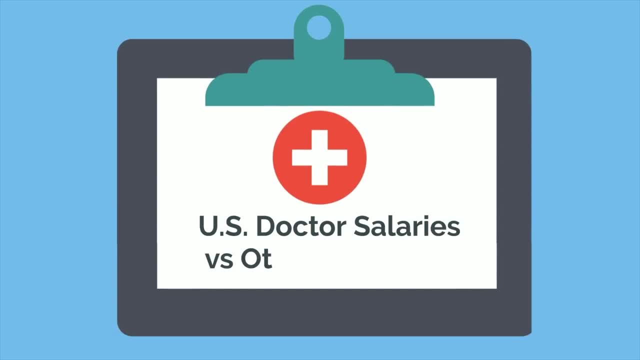 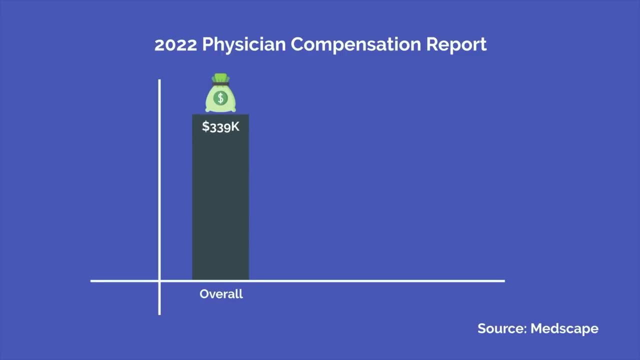 Let's start with the salary for US physicians compared to other countries. According to Medscape's 2022 Physician Compensation Report, the average physician in the United States earns approximately $339,000 per year. If we break this down further, the average physician in the United States earns approximately $339,000 per year. 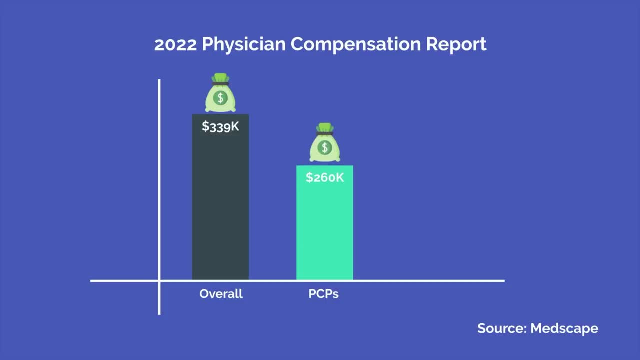 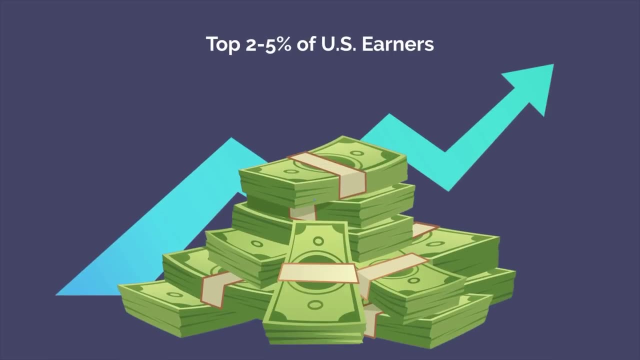 The average primary care physician earns approximately $260,000 and the average specialist earns $368,000.. This puts physicians in the top 2-5% of US earners. It should be noted that physician compensation in the US varies widely, both within and between. 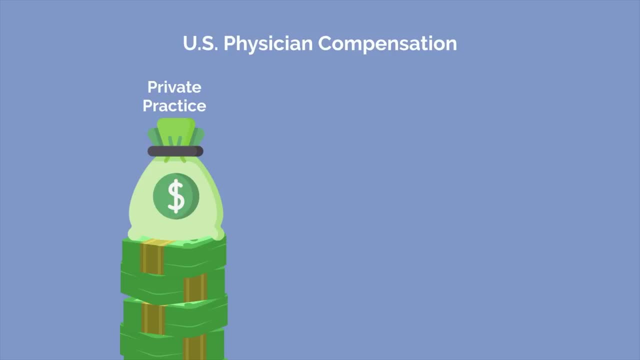 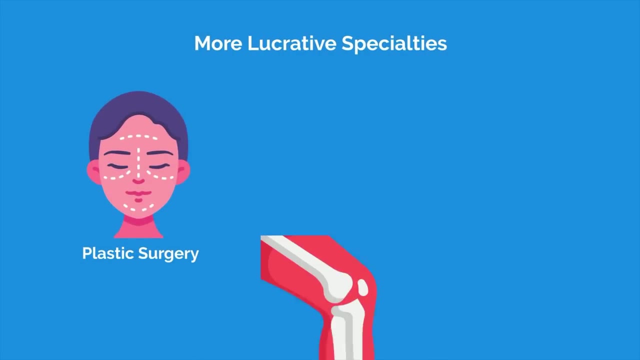 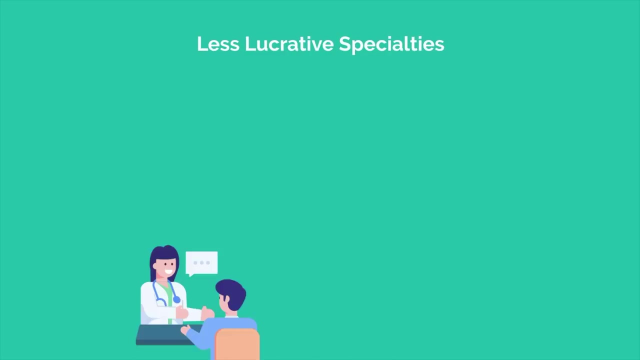 specialties. For instance, doctors working in private practice can often earn significantly more than physicians working in community or academic centers. In addition, more lucrative specialties such as plastic surgery, orthopedic surgery and cardiology can easily earn upwards of $500,000 per year, whereas less lucrative specialties such as family medicine and 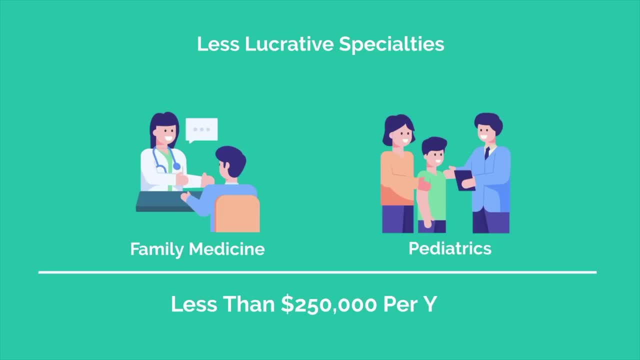 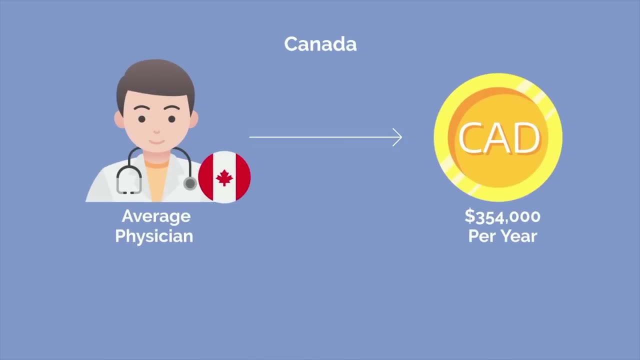 pediatrics may earn significantly less than that. Now let's compare these numbers to doctors in other countries. In Canada, the average physician earns approximately $354,000 per year. If we convert this to US currency, this is approximately $255,000, which is roughly $84,000 less per year. 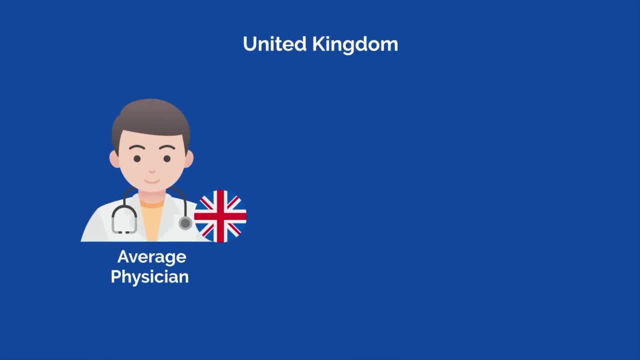 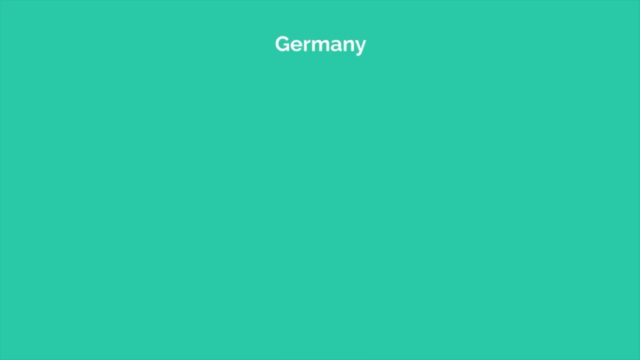 than the average US physician. In the United Kingdom, the average physician earns $107,000 per year, which equates to approximately $115,000 per year, And in Germany, the average physician earns roughly 93,000 euros, which currently equates to about $90,000.. As we can see from 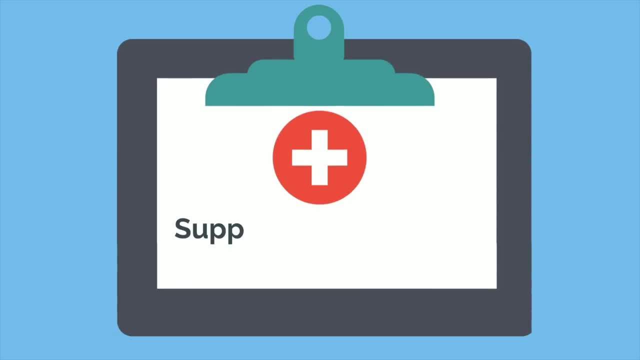 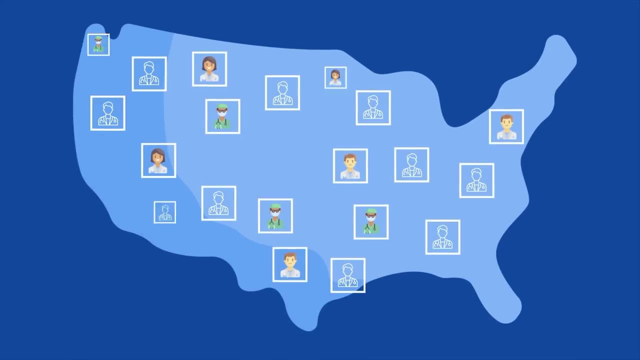 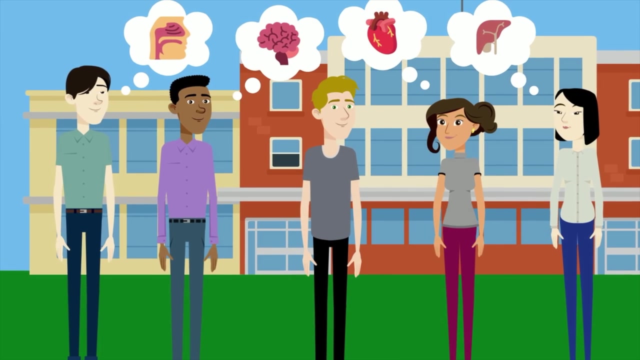 these numbers, US physicians are paid substantially more than physicians in many other wealthy countries. Another argument in favor of American doctors being overpaid is that the physician shortage has been artificially inflated. There is no shortage of people who want to become doctors. Rather, there are systems in place that have limited the number of physicians who want to become doctors. 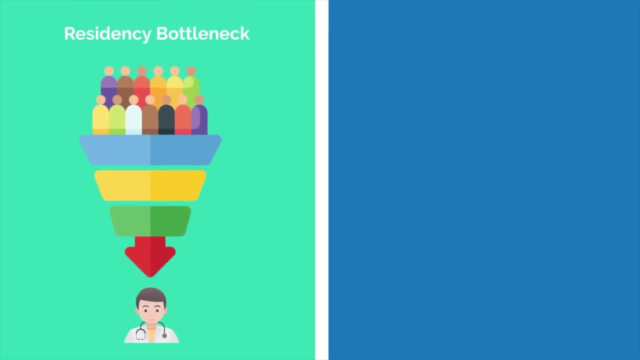 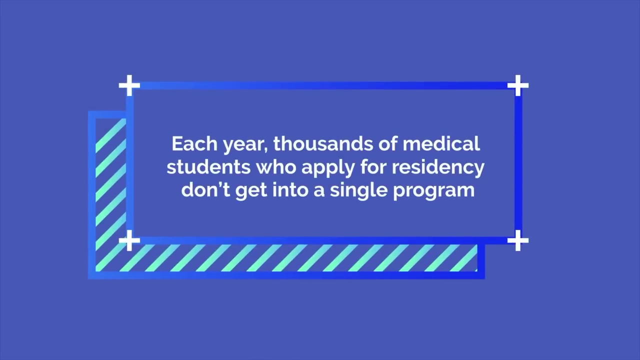 They have limited the number of physicians that can be trained each year, the most notable of which is the residency bottleneck. This, in turn, has inflated physician salaries. Each year, thousands of medical students who apply for residency don't get into a single program. 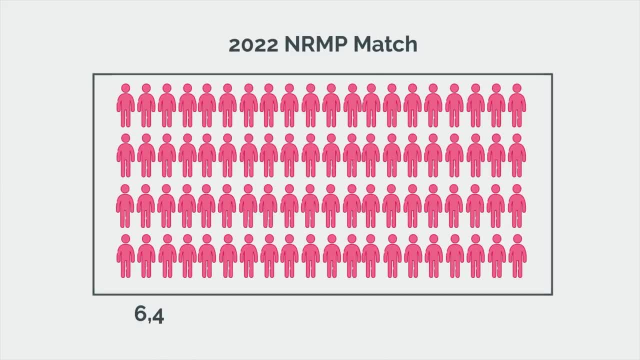 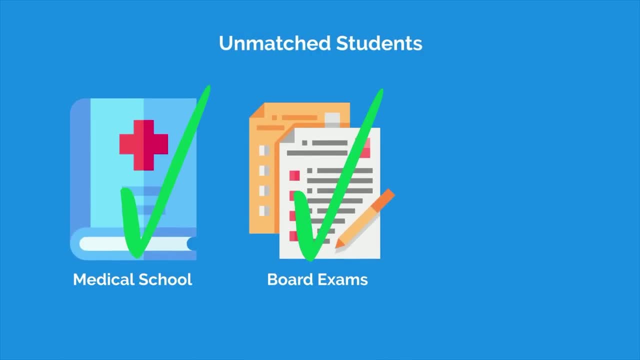 During the most recent 2022 NRMP match, approximately 6,400 students went unmatched. These are individuals who have completed medical school, passed their board exams and demonstrated that they have what it takes to be a doctor, and yet they are unable to continue their training. 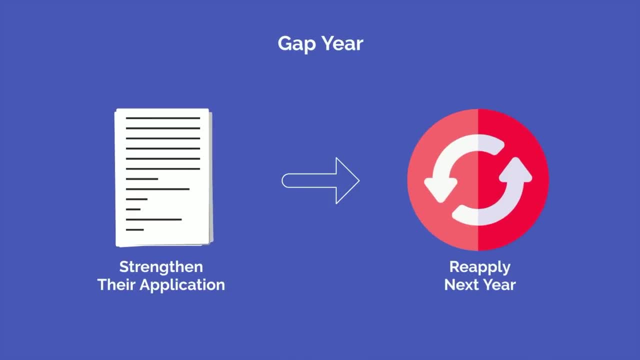 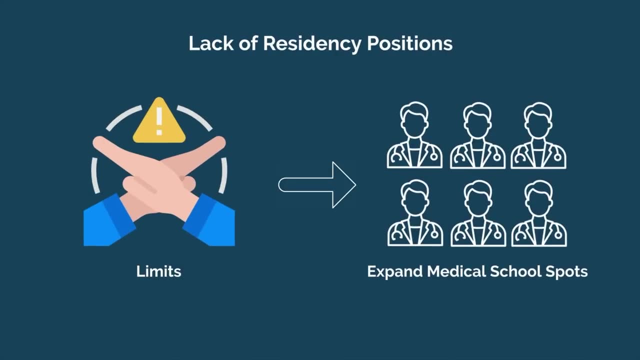 The gap year to strengthen their application and reapply in hopes of getting in next year. This lack of residency positions then trickles down and limits our ability to expand medical school spots as well. The reason that there aren't enough residency spots is due to the 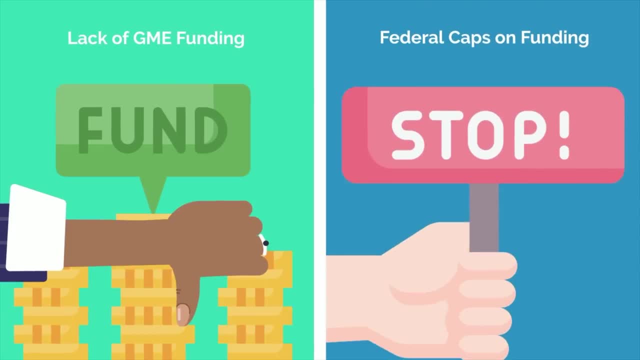 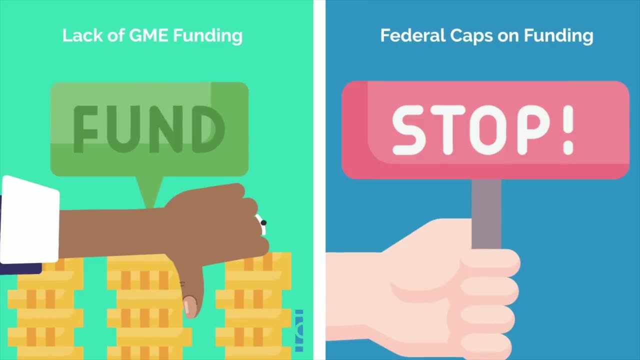 lack of Medicare, Graduate Medical Education or GME funding. Caps on funding imposed in 1997 have severely limited the number of facilities eligible to receive federal funding, making it much harder to open new residency programs. This is slowly changing with the recent 2021. 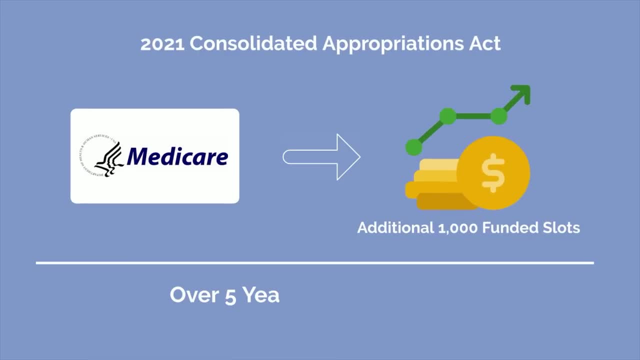 Consolidated Appropriations Act, which will have Medicare provide an additional 1,000 funded slots over 5 years, starting in 2023.. However, there will still be thousands of students who go unmatched each year. By limiting the number of physicians that can be trained each year, the United States 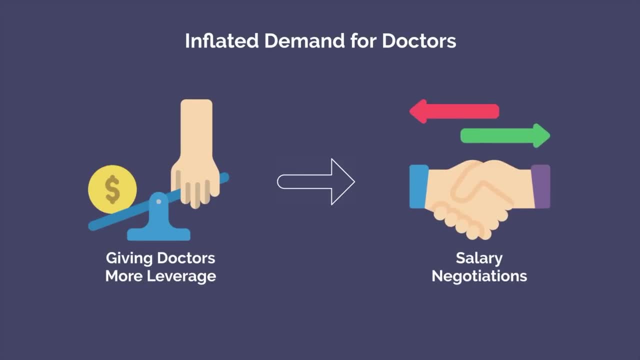 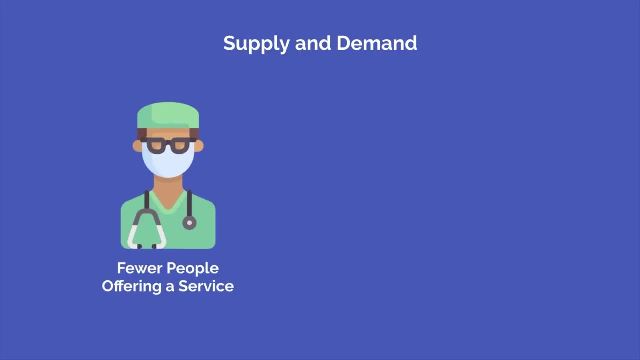 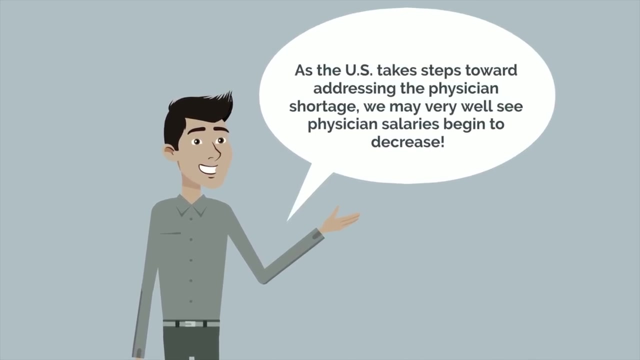 has artificially inflated the demand for physicians, giving doctors more leverage in salary negotiations. This has substantially driven up salaries. It's simple supply and demand. If there are fewer people offering a service, they can often charge more for that service. For this reason, as the US takes steps toward addressing the physician shortage, we may very well see. 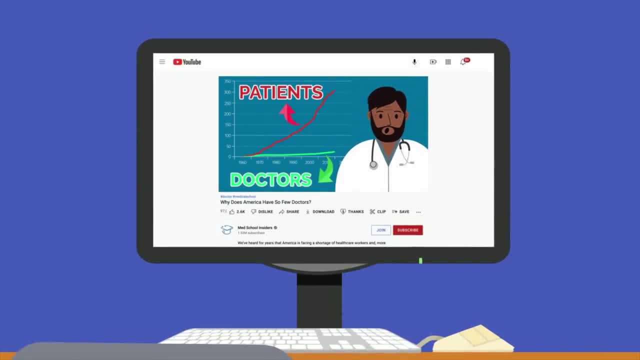 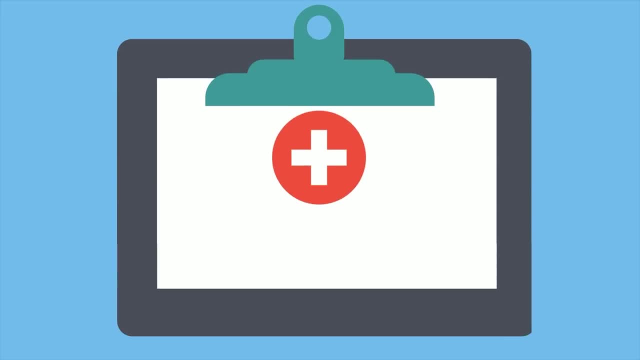 physician salaries begin to decrease. To learn more about the issues of physician shortages in the United States, be sure to check out. Why Does America Have So Few Doctors? link in the description. Lastly, some people argue that many of the responsibilities of a physician can be. 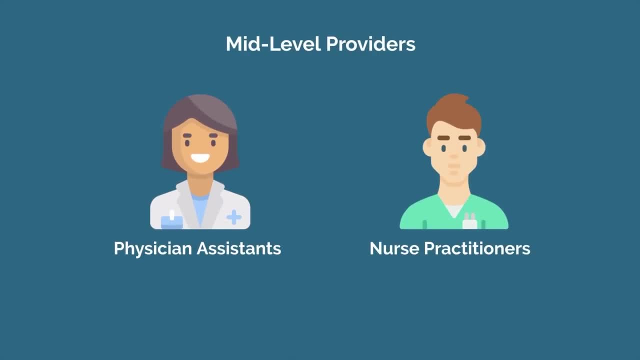 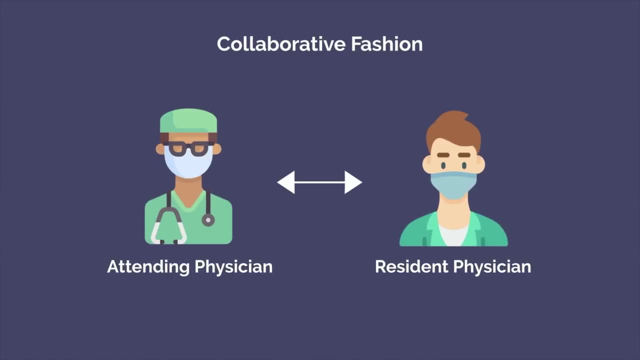 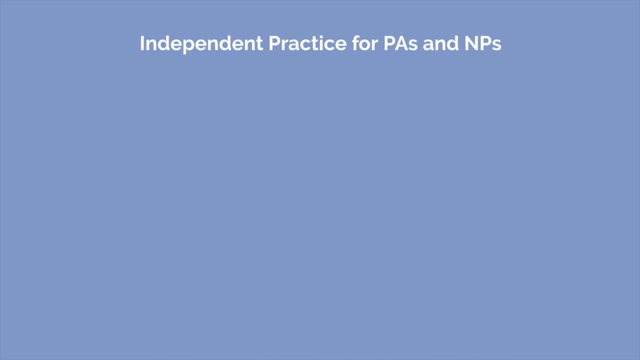 accomplished by mid-level providers, such as physician assistants and nurse practitioners, at a much lower cost. Traditionally, mid-level providers work in a collaborative fashion with doctors, similar to the relationship between an expert and a physician. As a result, the average physician in the United States earns approximately $339,000 per year. 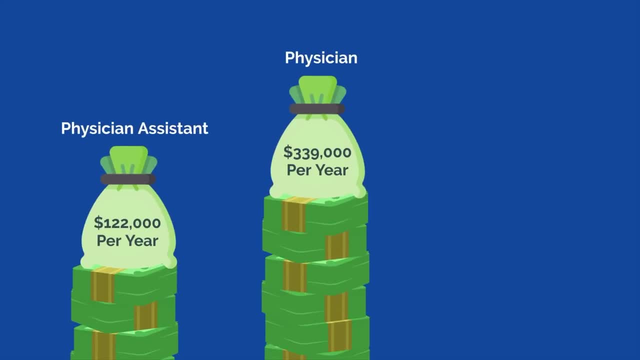 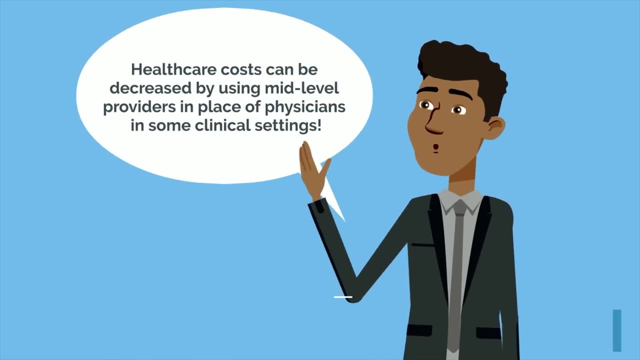 whereas the average PA earns $122,000 per year and the average NP $118,000 per year. This large gap in pay has led many to question if healthcare costs can be decreased by using mid-level providers in place of physicians in some clinical settings. That being said, 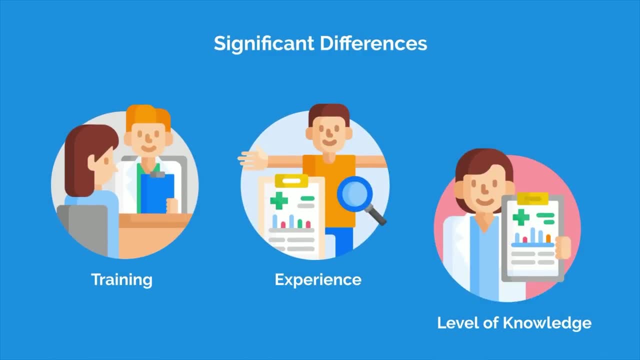 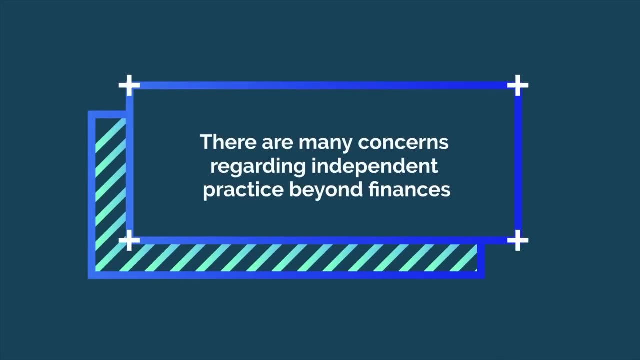 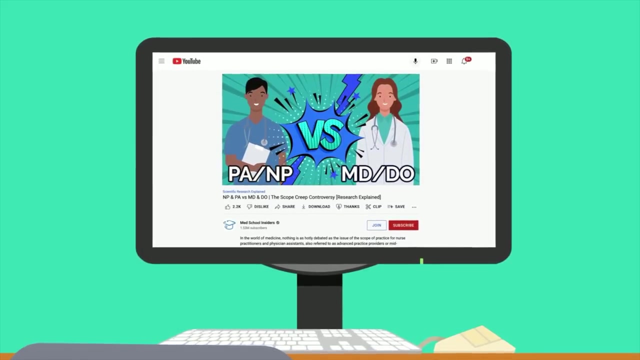 there are significant differences in the training, experience and level of knowledge between physicians and mid-level providers. As such, there are many concerns regarding independent practice beyond finances. That discussion, however, is beyond the scope of this video. For a comprehensive overview of the independent practice debate, be sure to check out our NP and 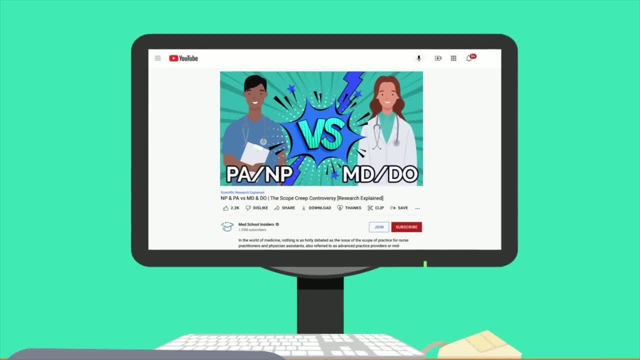 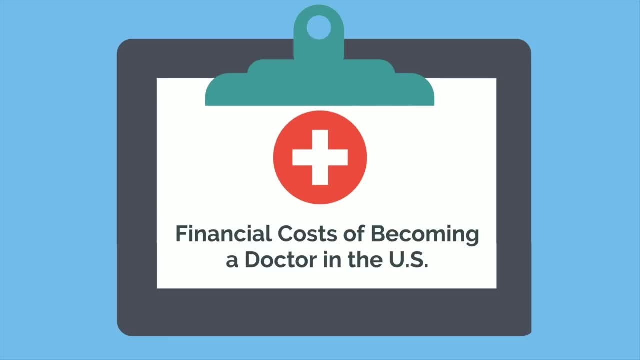 PA vs MD and DO comparison video link in the description. Now let's get into the arguments between the two. The first is the cost of being a doctor. The cost of being a doctor in the United States is incredibly expensive. Before starting medical school, you must first complete a four-year. 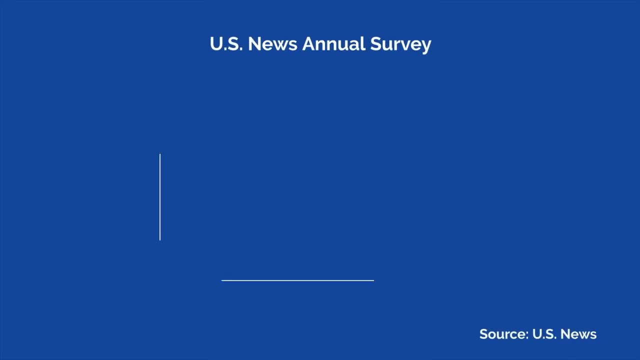 bachelor's degree. According to a US News annual survey, the average cost of college tuition per year in 2022 was $40,000 for private colleges, $23,000 for out-of-state students at public schools and $10,000 for in-state residents at public colleges. This means that it costs students. 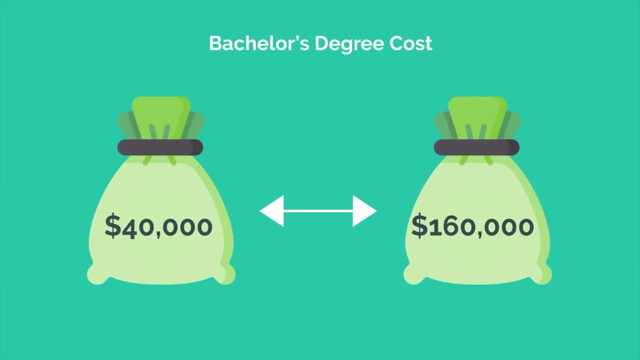 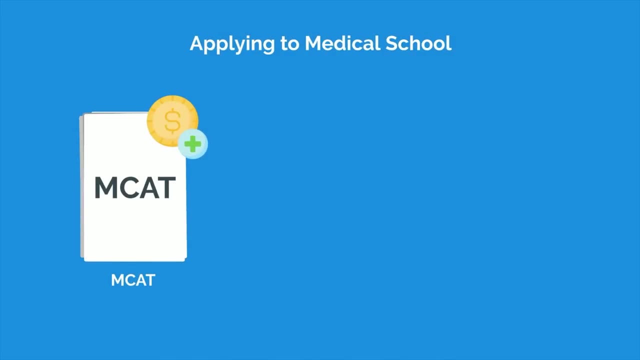 anywhere from $40,000 to $160,000 to earn their bachelor's degree, And these numbers don't take into account the various other fees associated with applying to medical school, including the cost of taking and sometimes retaking the MCAT, application fees and attending interviews. 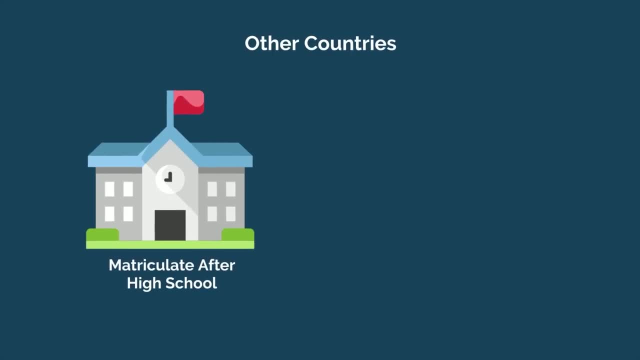 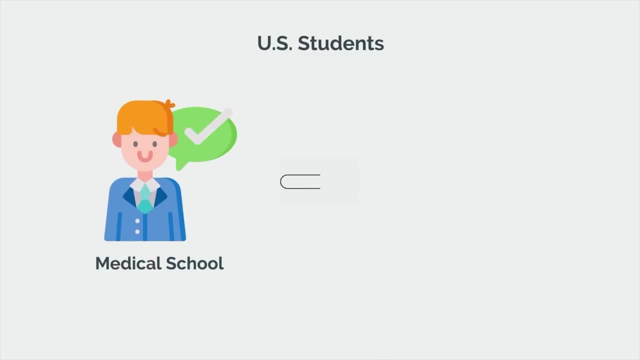 In contrast, many other countries allow students to matriculate into medical school straight out of high school, with some even offering free college tuition. Once US students gain admission to medical school, however, the costs escalate even further As of 2022,. 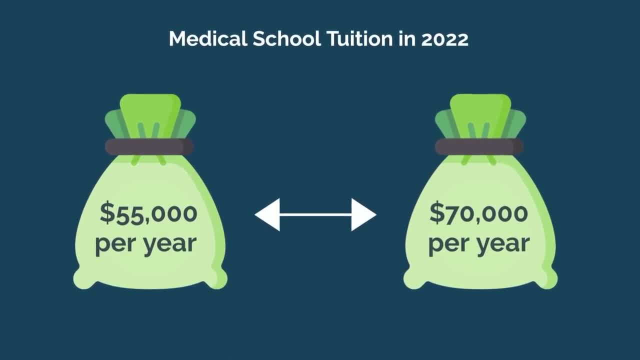 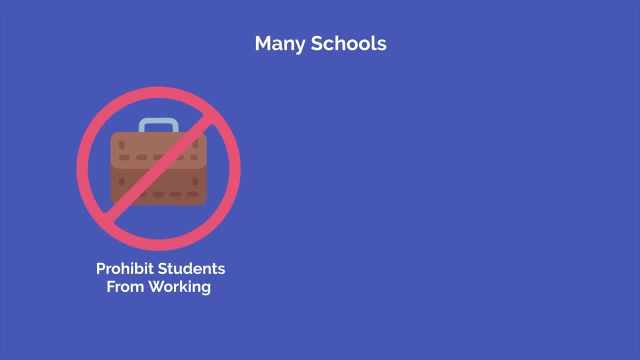 the average cost of medical school tuition in the United States is approximately $55,000 per year, with some schools charging more than $70,000 per year. In addition, many schools explicitly prohibit students- and for good reason- from working during medical school, making it. 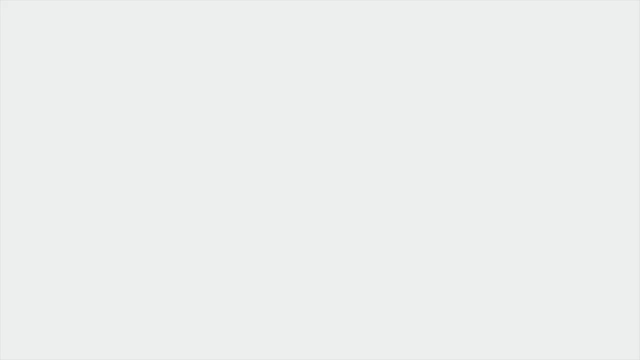 practically impossible to earn a livable income during these four years. As a result, the majority of students are forced to rely on loans to pay for school and other living expenses. It should come as no surprise, then, that the average medical student graduates with around 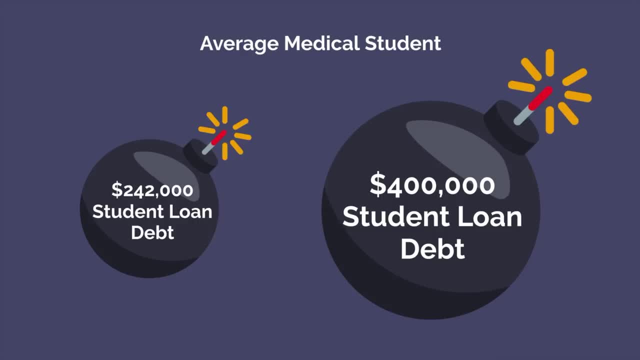 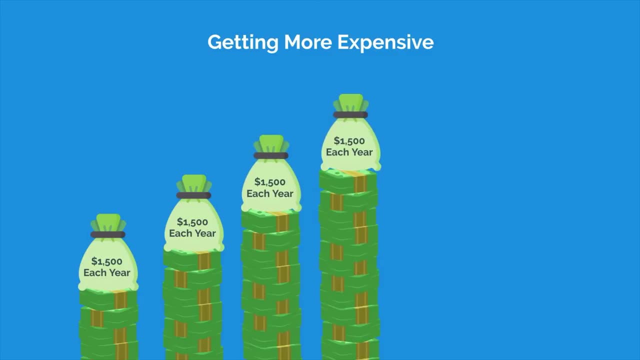 $2,000 of student loan debt, with some students owing over $400,000 by the time they graduate. It's only getting more expensive, too, as the average cost of medical school rises by approximately $1,500 each year. During residency, US doctors will begin earning a salary. However, it is not. 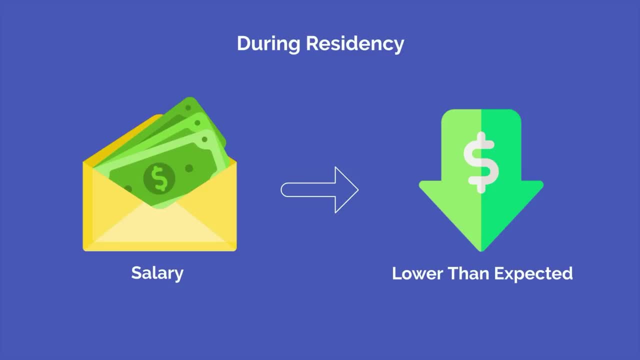 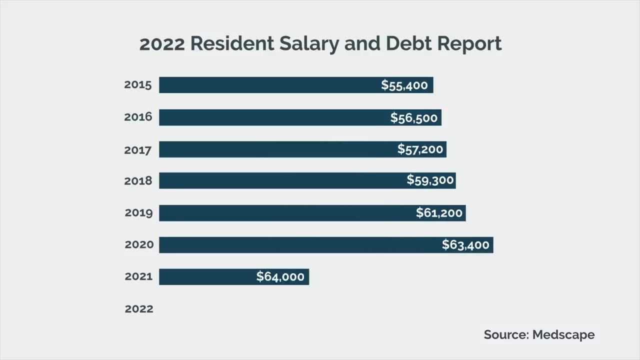 as much as you might expect for someone with over 8 years of post-secondary education. According to Medscape's 2022 Resident Salary and Debt Report, the average salary for residents in 2022 was approximately $64,000.. The average salary for residents in 2022 was approximately $64,000. 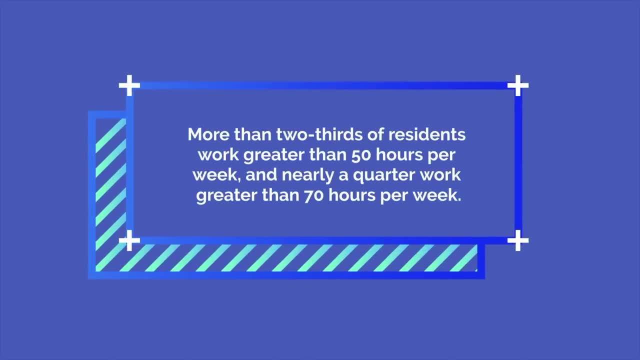 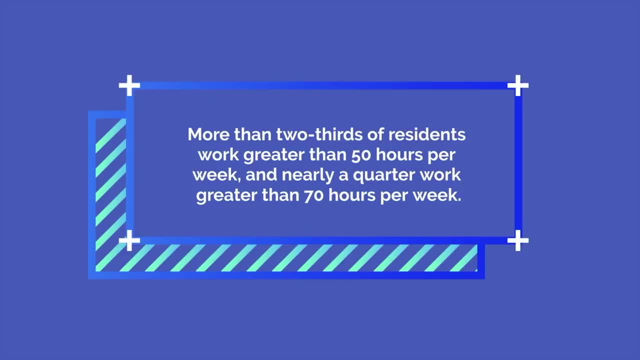 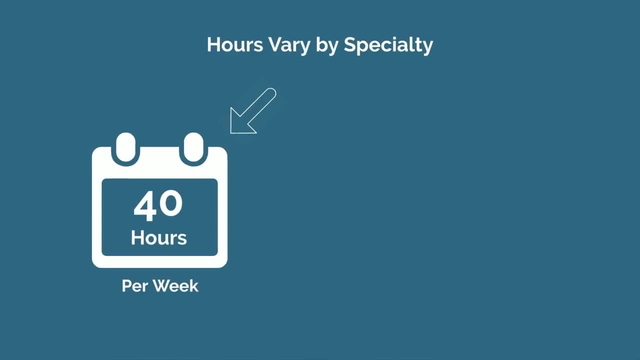 work greater than 50 hours per week and nearly a quarter work greater than 70 hours per week. This varies widely based on specialty, however, with some specialties averaging close to 40 hours each week and others more than 80 hours per week. Although duty hour restrictions exist, that limit 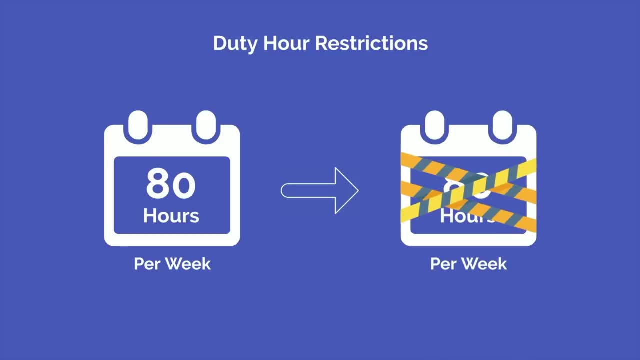 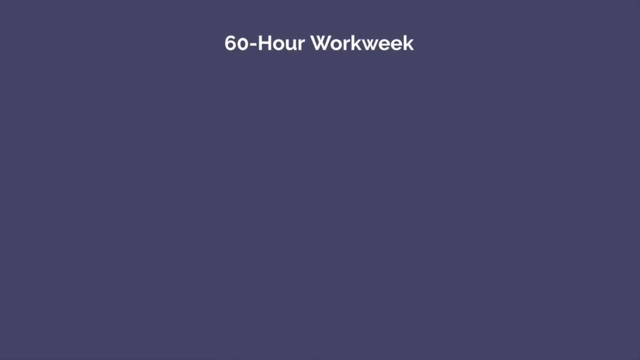 residents to working no more than 80 hours per week. many programs violate these restrictions. If we use a modest estimate of a 60-hour work week, the average resident physician earns a approximately $21 per hour after nearly a decade of training and accruing between a quarter to half. 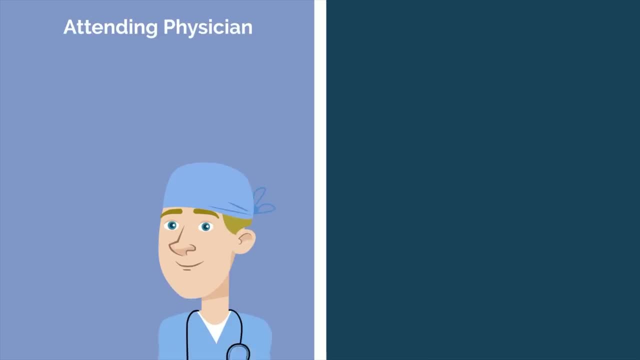 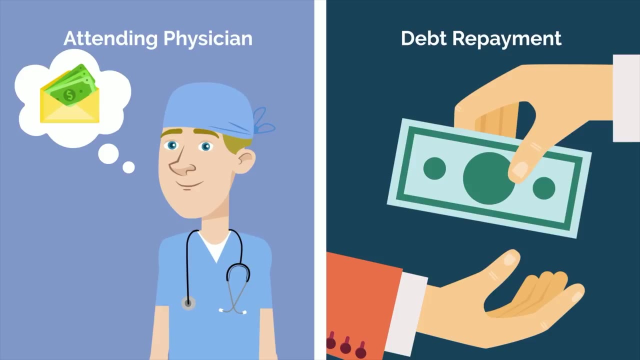 a million dollars of debt. Although salaries increase significantly once a resident becomes an attending physician, they are often well into their 30s by this point and will then have to start the long road of debt repayment. This brings us to the next point, which is the significant. 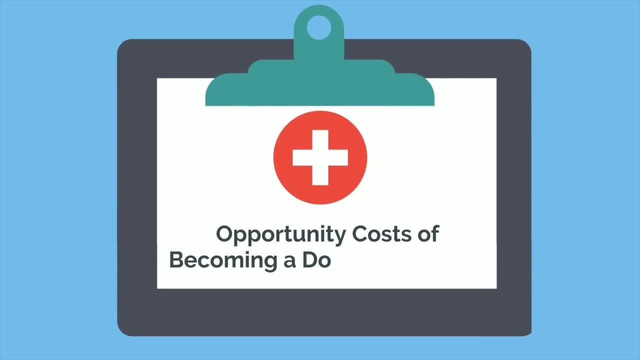 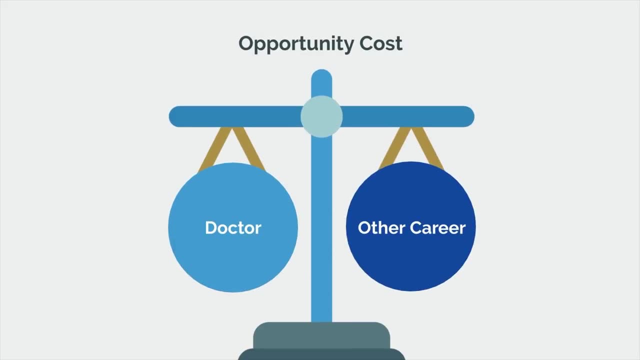 opportunity cost associated with becoming a physician. in the US. Opportunity cost can be defined as the potential loss from a missed opportunity resulting from choosing one alternative over another. To start, it takes a minimum- a minimum of 11 years after high school to become a doctor in the United States. That's four years. 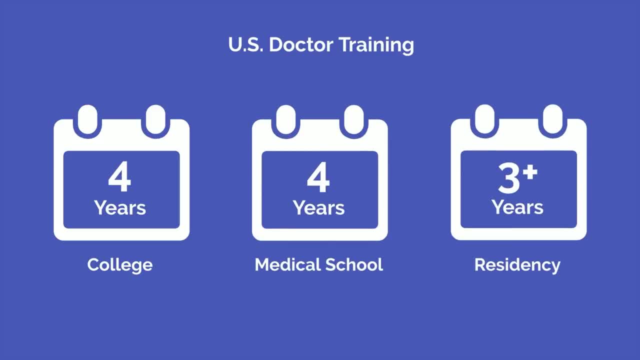 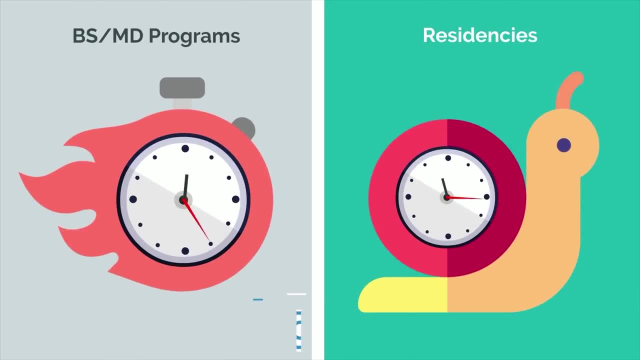 of college, followed by four years of medical school and three years of residency. Although there are some pathways that can shorten the length of training slightly, such as BSMD programs, these are not the norm. In addition, many specialties have residencies lasting longer. 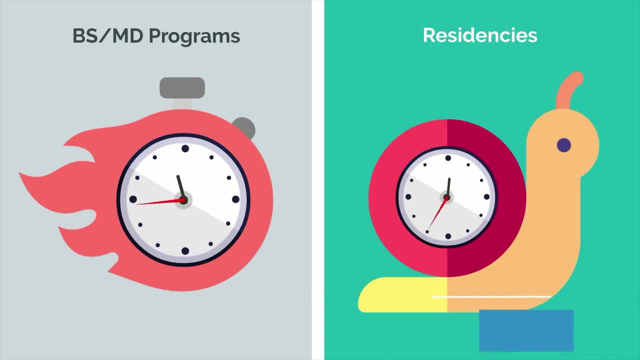 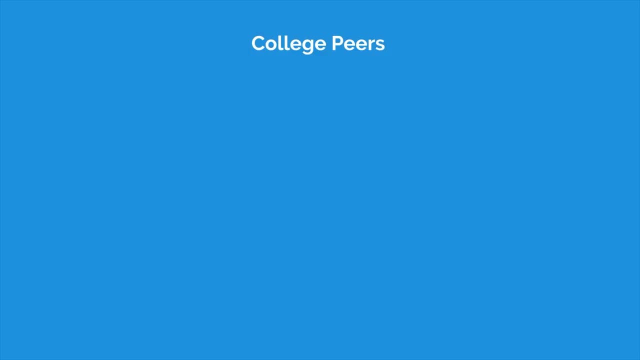 than three years, and that's not even getting into the various fellowships available. Physicians spend over a decade of their lives in training before they start their careers. In comparison, many of their college peers will complete their four-year degree and begin their desired field and begin climbing the career ladder. As such, they will have nearly 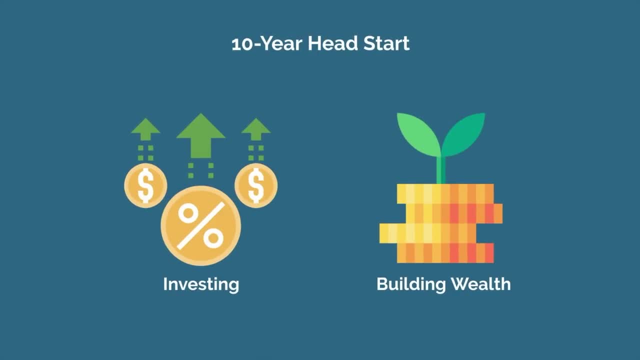 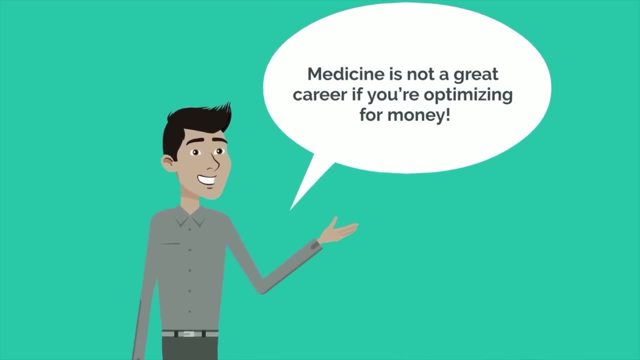 a decade's head start in terms of investing and building their wealth. This is why I have said many times on this channel that medicine is not a great career if you're optimizing for money. If you do want to optimize for money, however, I have an entire video discussing the highest-paying. 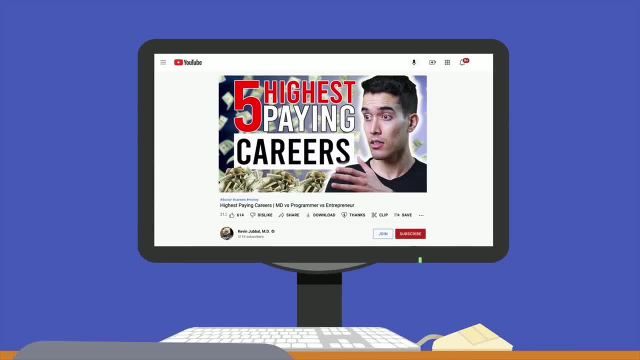 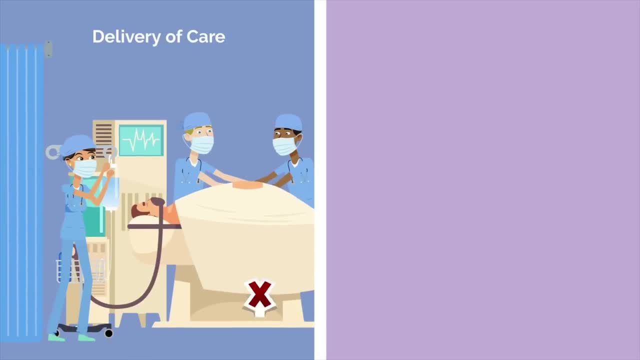 careers over on the Kevin Jubbal MD channel link in the description. The last argument against American doctors being overpaid is that they aren't actually the highest earners within medicine. The real money in medicine is not in the delivery of care, but rather in overseeing the business of medicine. According to a New York Times survey,